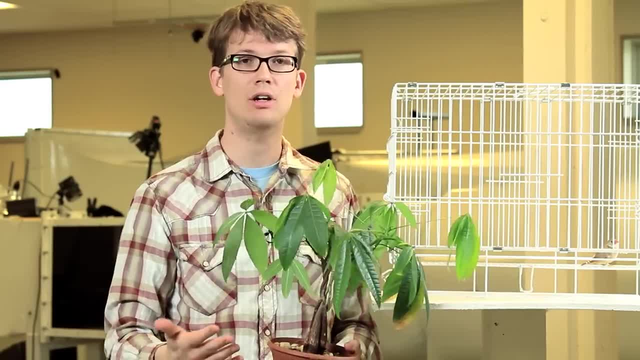 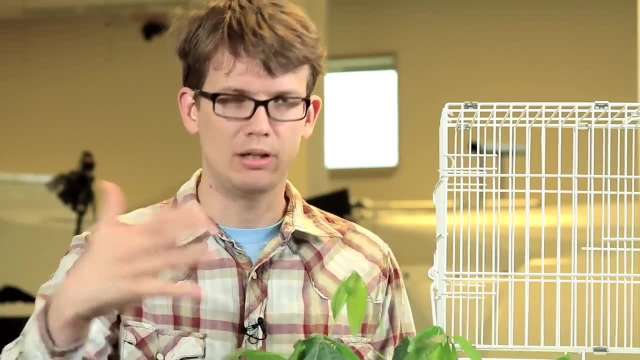 While Shoshanna can't make her own food, she has to move around to find stuff to eat, to escape predators, to find mates, to poop on park benches- Just like me, Except not the pooping on park benches. I mean the pooping on the park benches. Just like me, Except not the pooping on park benches. I mean the pooping on the park benches. 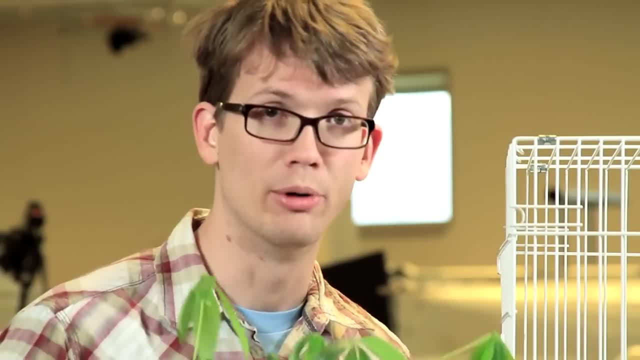 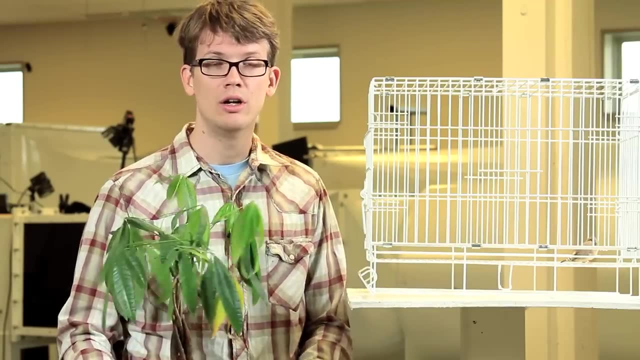 the moving around. So yeah, shocker, I am more closely related to a bird than to a plant. You get a gold star, So that one's obvious. but as the relationships between organisms get closer, the questions get a lot more interesting. So what is an animal? I mean, I know, you know. 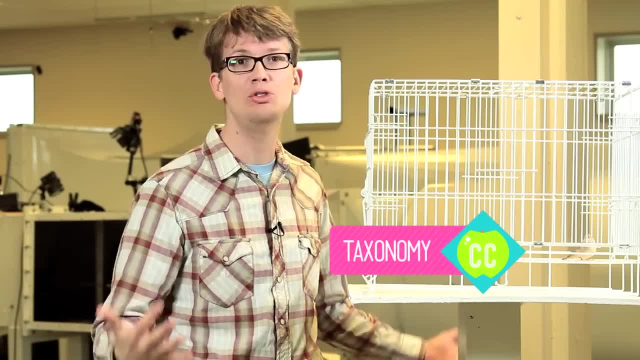 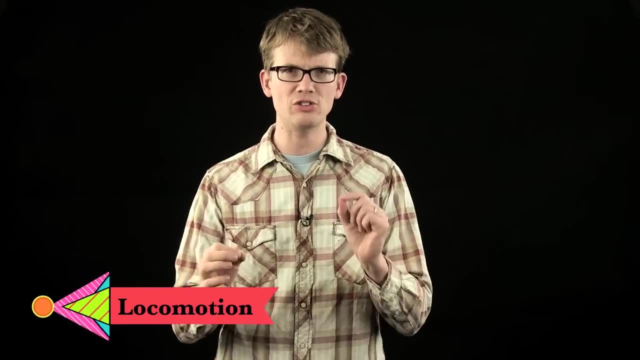 what an animal is. but when you're looking at Shoshanna and me here, what clues you aid in to the fact that we are members of the kingdom Animalia? Two things, For starters: we're both moving. Locomotion is a really good sign that an organism is an animal, unless 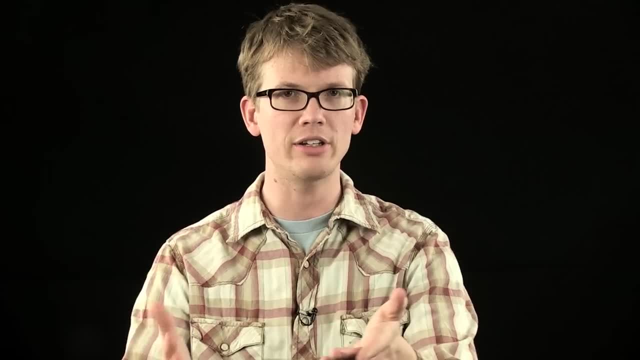 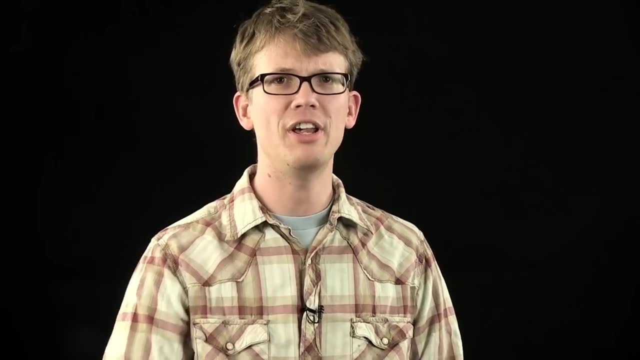 you're a sponge, I know what you're thinking, though. Protists, bacteria and archaea, they all move around using flagella and cilia, but they also only have one cell. It's the multicellular locomotion that's so peculiar and specific to animals. So animals move because 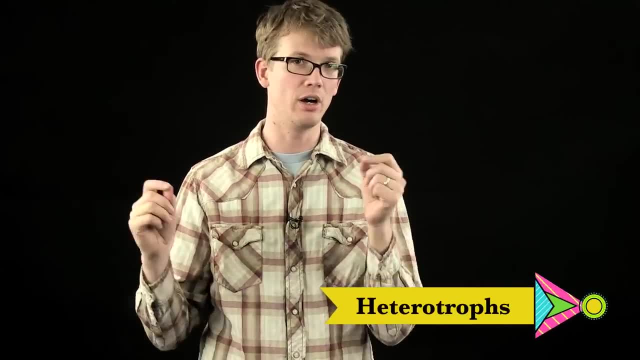 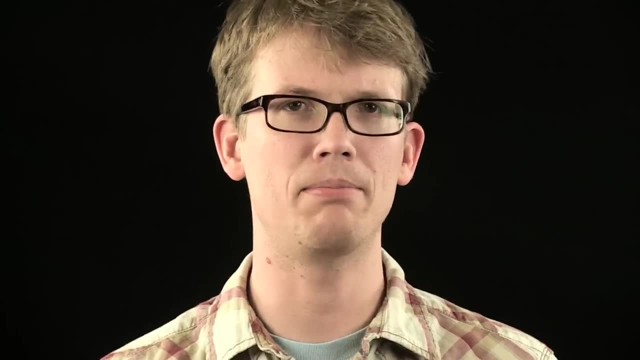 of the second trait that we have in common: We're heterotrophs. We get our energy from eating other life forms. Locomotion also helps us avoid predation and seek out mates for reproduction. Now plants. they can mate by dispersing their seed to the wind or having 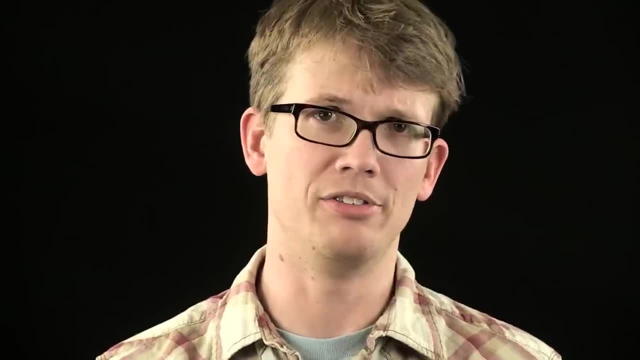 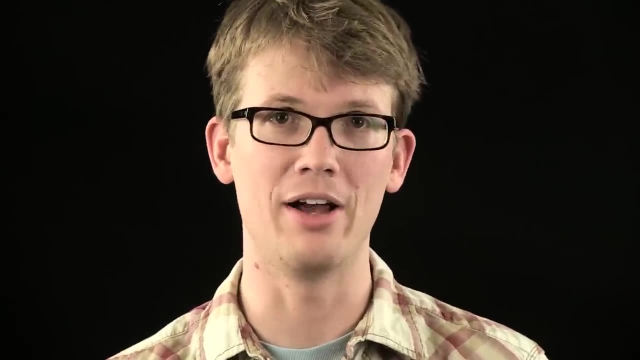 an insect come by and fertilize them. But if land animals did that, things would get like really messy and gross. Some aquatic animals actually do: just release their sex cells into their surroundings and cross their fingers and presumably close their mouths and hope that somebody gets pregnant. So since 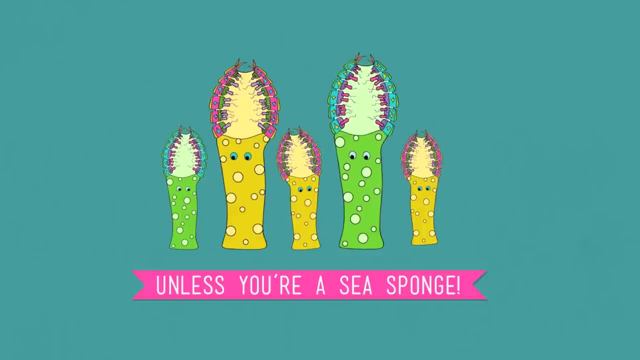 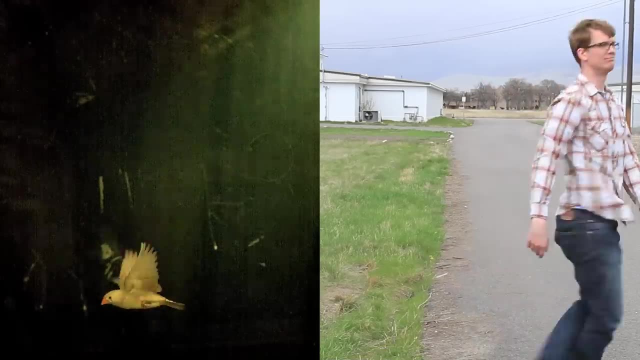 animals have to eat and move around. they've evolved anatomical forms that help them do those things, But obviously those forms aren't the same in all animals. For instance, in order to move, Shoshanna and I both have to be able to apply force to the ground or the 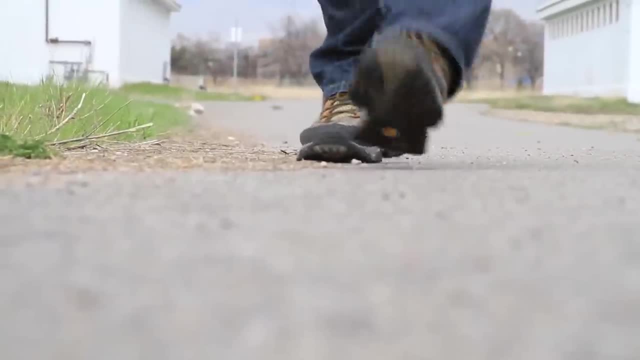 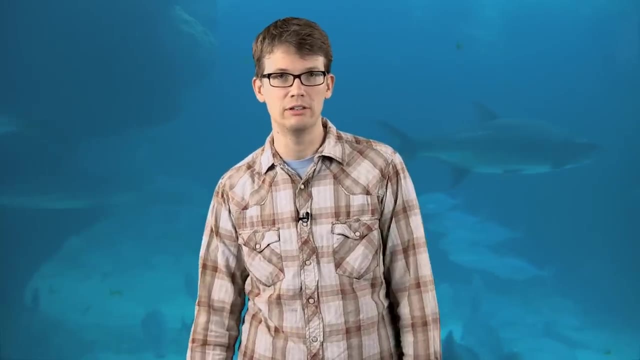 air to propel ourselves. Here is me pushing off the ground with my feet, And now here's Shoshanna applying force to the air with her wings which keeps her afloat and moving. And if I had a shark in the studio with me, which thankfully I do not, so I'll 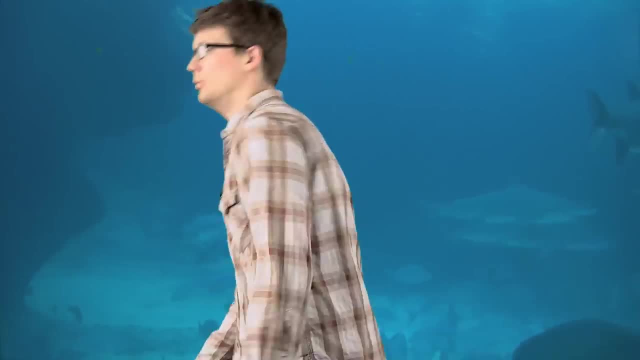 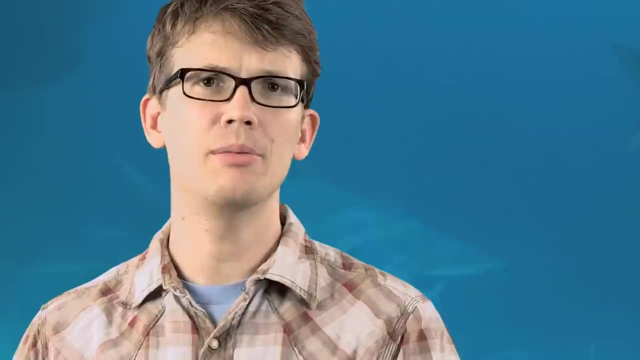 just pretend to be a shark. my fins would apply force to the water, which would propel me forward. I have to be careful with this stuff because even though similar body structures like fins or wings or feet can mean animals have a close common ancestor, it can also mean that the 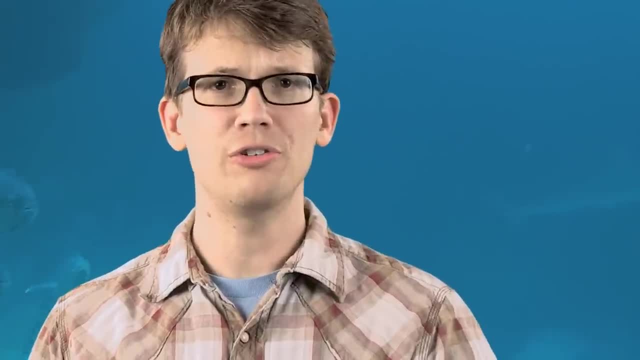 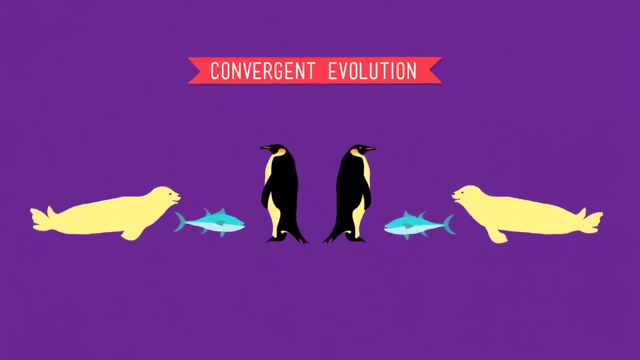 animals just evolved similar forms, because that's the best structure for the job. When this happens, it's called convergent evolution. For example, a tuna, a penguin and a seal are all animals that spend all or a lot of their time in the water. One's a fish, one's 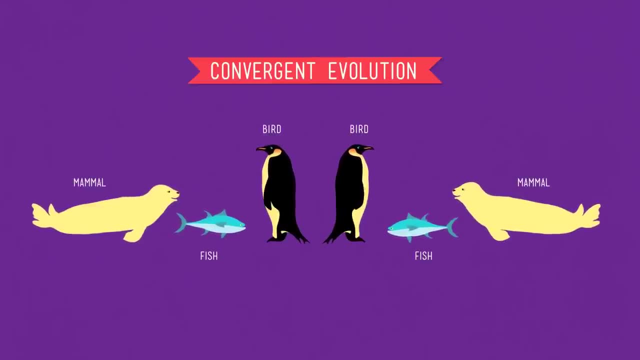 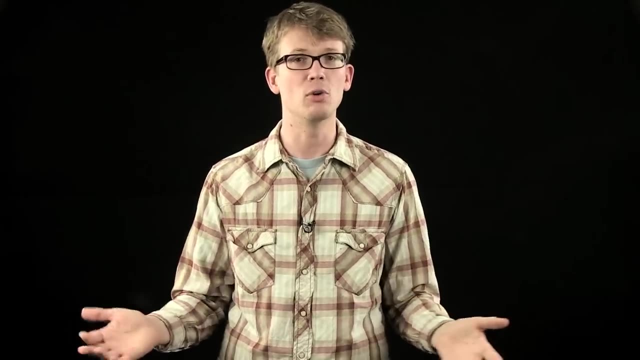 a bird, one's a mammal, but all three of them have a suite of similar features, the most notable being a really sleek fusiform body that can move through the water like nobody's business, and fins for propelling those bodies. 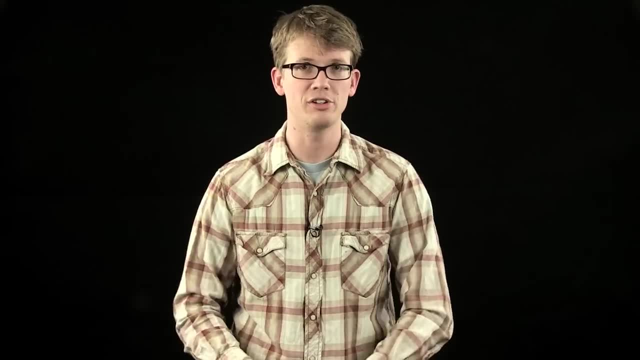 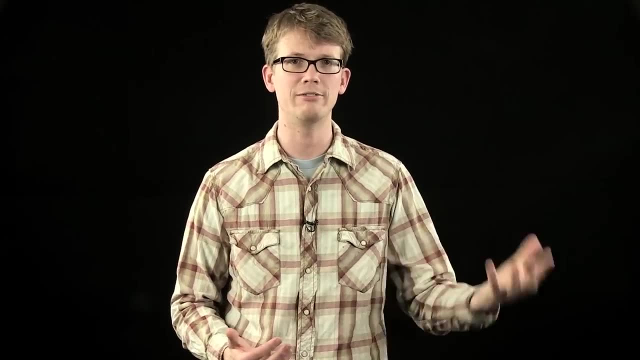 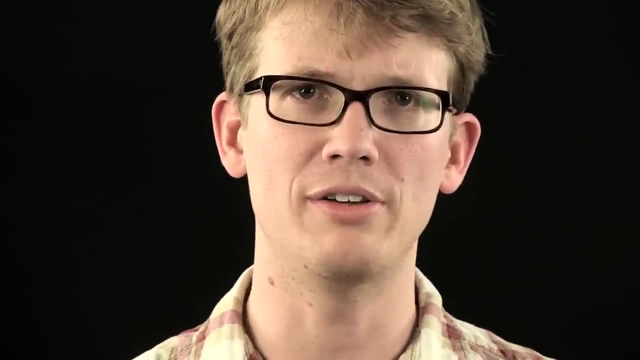 But of course those three animals have very different evolutionary origins. Each of these three marine animals have independently converged on similar body shapes because they live in the same environment and need to do the same sorts of things. So instances of convergent evolution can make linking physical structure of an animal to its evolutionary history a 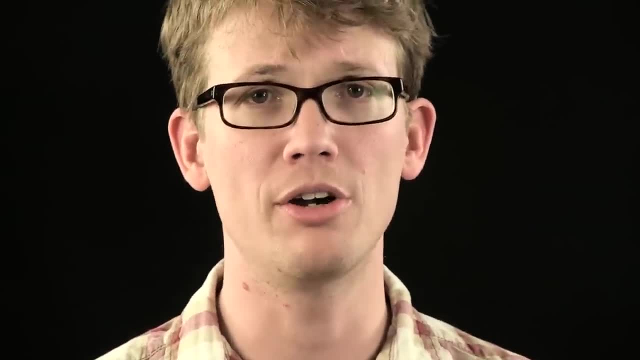 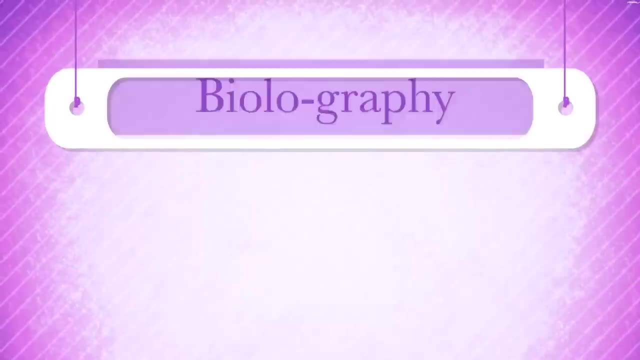 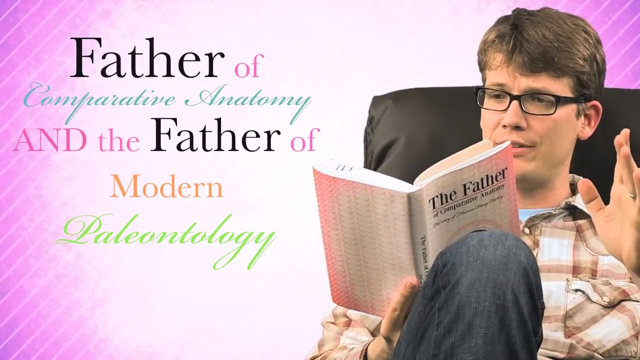 little bit tricky, which is why for a long time, nobody really put much stock in comparative anatomy as proof of evolution. That is until Thomas Henry Huxley came along. Thomas Henry Huxley was the father of comparative anatomy and the father of modern paleontology. 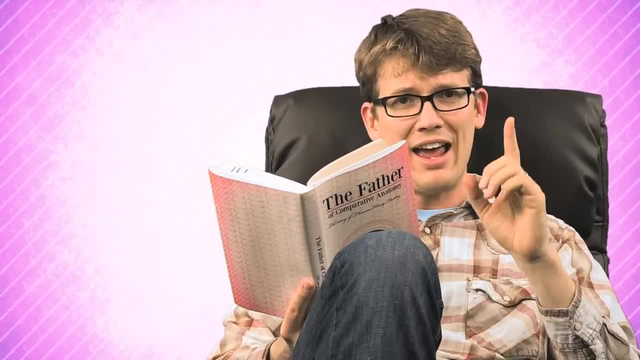 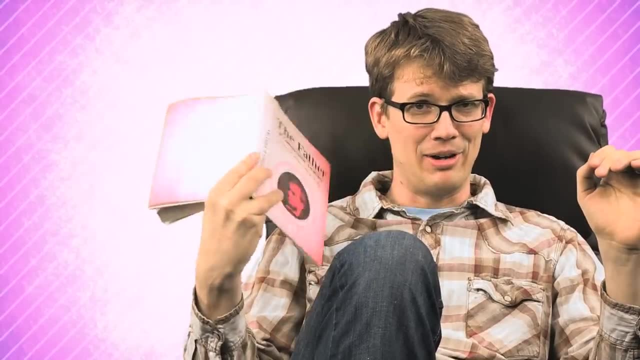 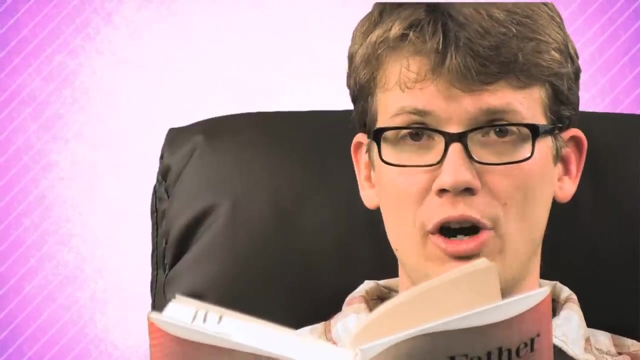 and he invented the word agnostic to describe his spiritual views, and he was the first to conclude that birds evolved from small carnivorous dinosaurs. I'm glad I'm sitting down for this. Plus, we have much respect for his facial hair. Huxley was born in England in 1825 and though he started out as a doctor after serving as 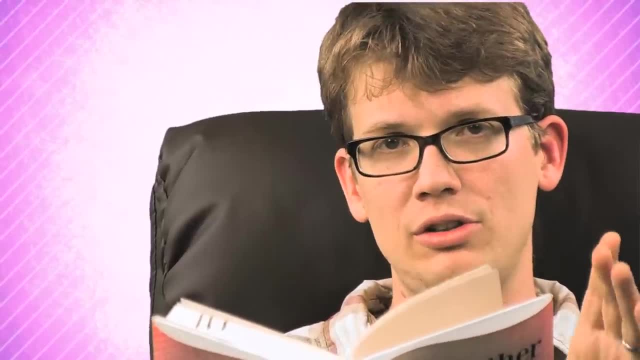 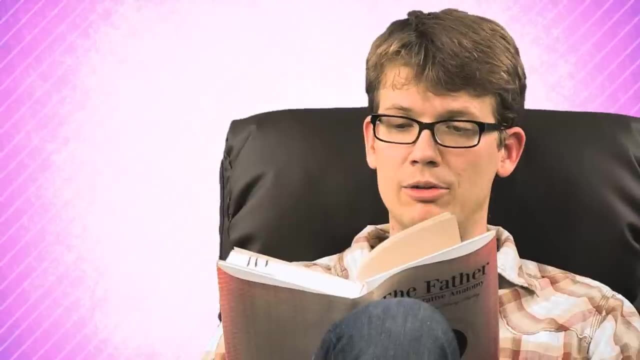 a ship surgeon. on a voyage to Australia in his twenties he took to studying marine invertebrates. During his voyage he sent all of his papers back to England and when he got home he found that he had become a kind of famous marine invertebrate expert and he was admitted into 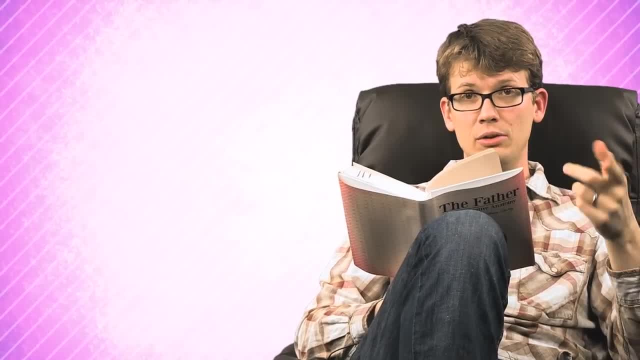 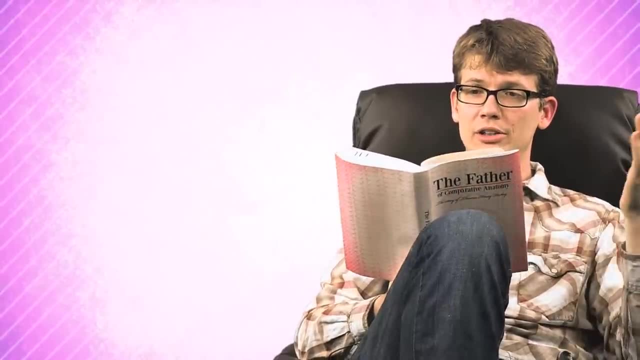 the Royal Society, Huxley made friends with some other hotshot natural scientists, including Charles Darwin, and a few years later, when Darwin outlined his theory of evolution and on the origin of species, Huxley is reported to have said: How extremely stupid not to have thought of that. 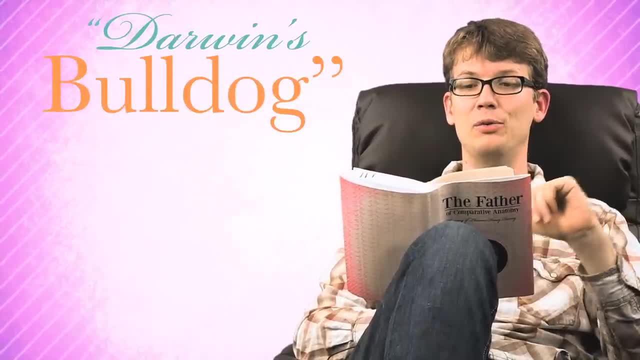 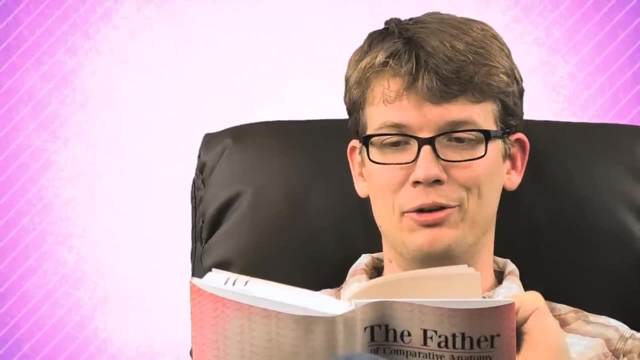 In fact, he became such a huge Darwin supporter that everybody started calling him Darwin's bulldog, because he threatened to cut the fool who badmouthed evolution. This is a good one, Huxley said when he was talking about On the Origin of Species. 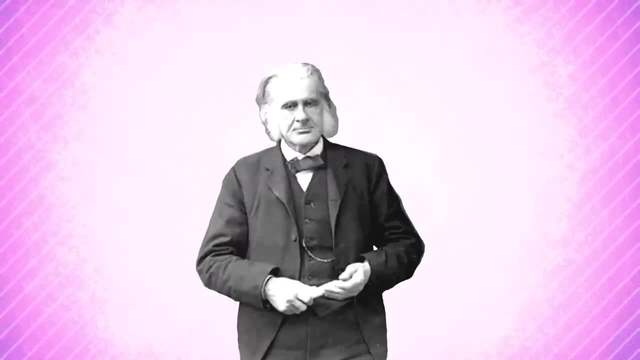 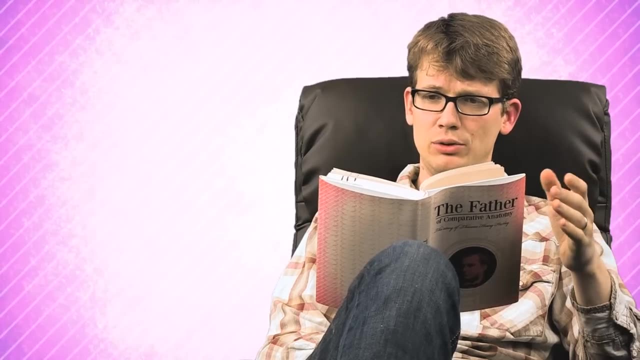 Old ladies of both sexes consider it a decidedly dangerous book. You just got Huxlapped With this new tool of the theory of evolution and in part to help promote the theory of evolution, Huxley connected paleontology and biology together by looking for similarities. 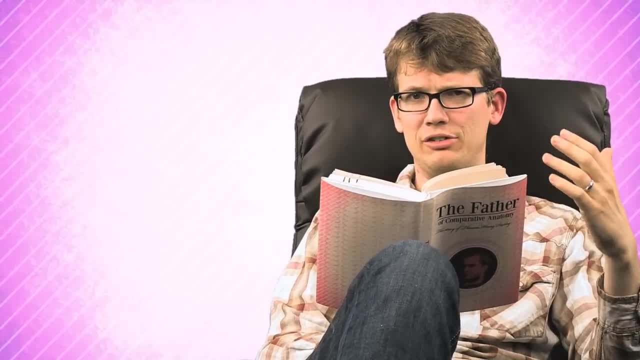 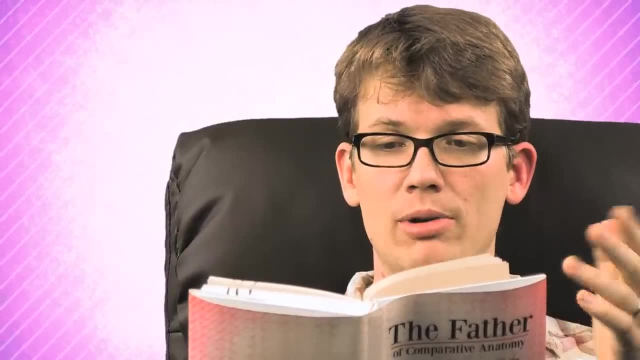 in anatomy, in the fossil record, where he found all kinds of interesting stuff, like some really obvious similarities between prehistoric horse fossils and modern day horses, as well as between dinosaurs and birds, though nobody really bought his insights into the resemblance between birds and dinosaurs for another hundred years. 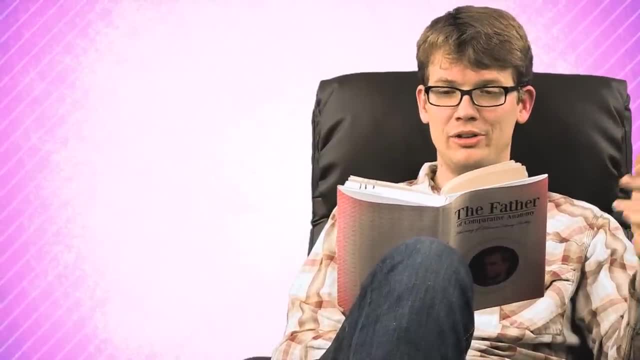 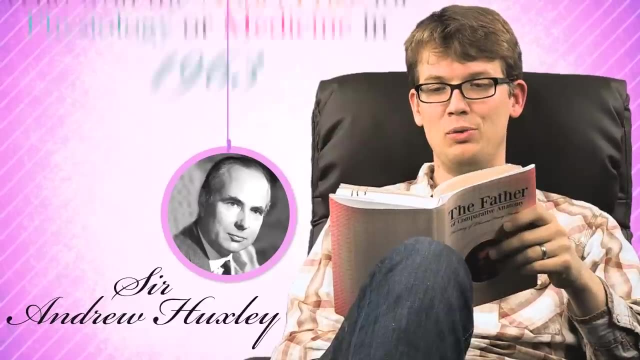 And just in case you were still on the fence as to whether intelligence is heritable, I'm sure Thomas Henry Huxley is the grandfather of brave new world writer Aldous Huxley and of Sir Andrew Huxley, who won the Nobel Prize for Physiology or Medicine in 1963. 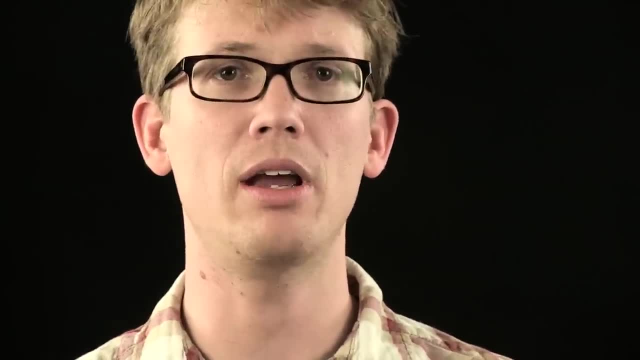 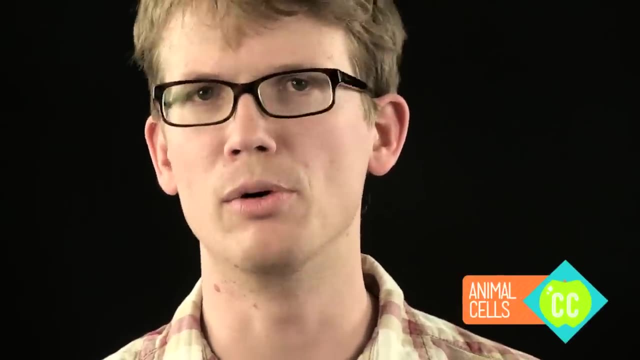 Because all animals come from the same evolutionary origin. in addition to sharing some anatomical structures, like Huxley studied, we're also built from the same rudimentary blueprint. Our cells work pretty much the same, no matter what sort of animal we are. 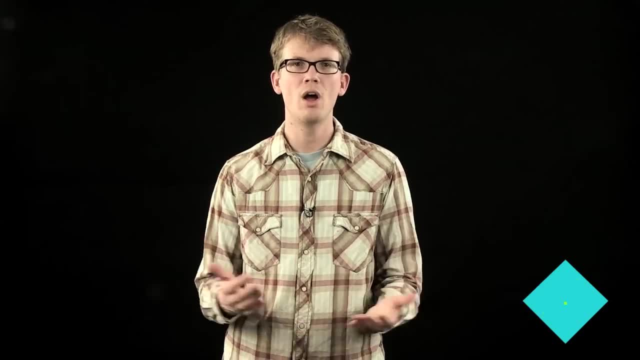 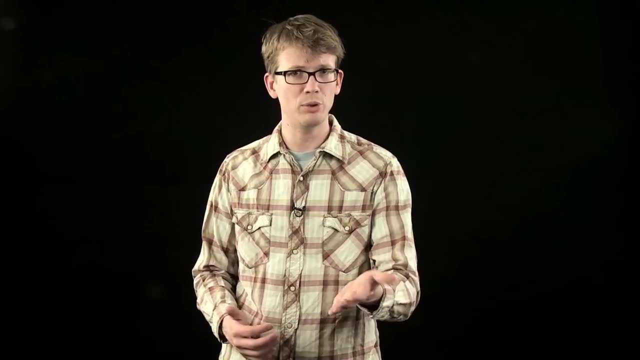 So while animals have different strategies for moving around and acquiring food, once the food is gotten, all animals break it down. They turn it into useful energy and distribute nutrients and eliminate waste in pretty similar ways. Unless you're a sponge, Each of those functions is performed by collections of cells that group together in the body to 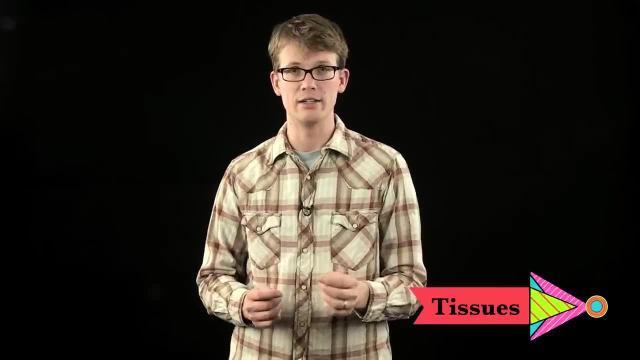 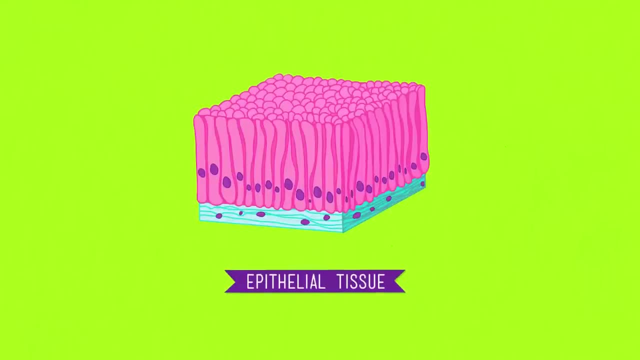 form tissues. There are four primary types of tissues in the human body: The epithelial tissue, the connective tissue, muscle tissue and nerve tissue. Epithelial tissue is formed by cells that bind very closely together. A layer of it covers every organ and lines the digestive tract to prevent crazy acids. 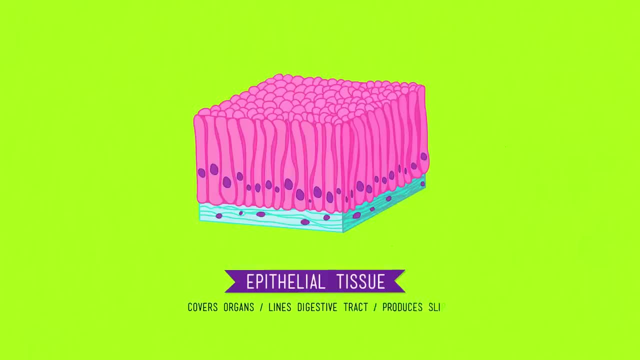 and poop and stuff from going where it's not supposed to go. The thrombocytopenia tissue is formed by a tissue that is put together by a tissue that is like a membrane that lines the inside of your ribs so that your inflating lungs don't. 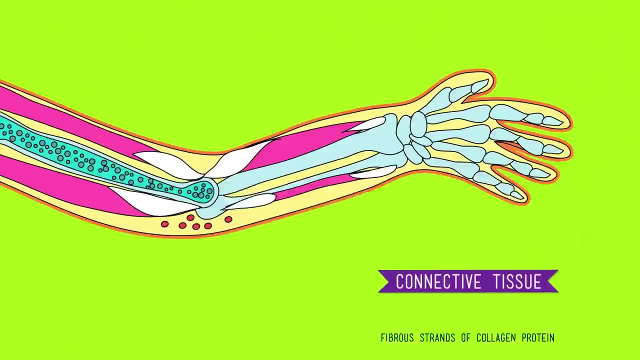 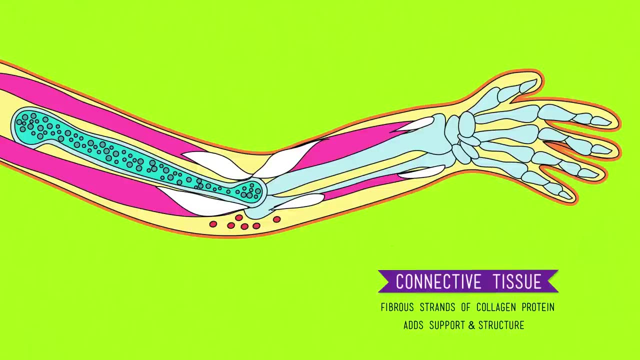 build up friction as they expand. Most types of connective tissue are made up of fibrous strands of collagen protein, and it adds support and structure to your body and holds your parts together. Some examples of connective tissue include the inner layers of your skin, your tendons. 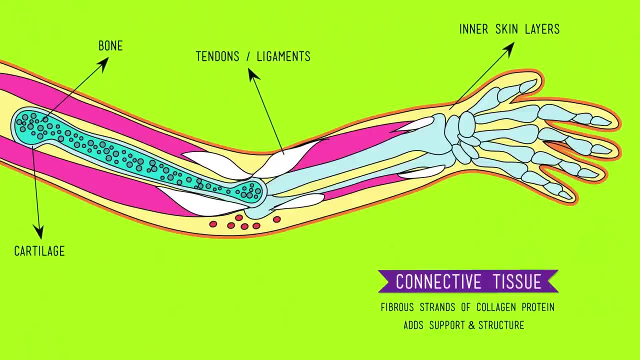 ligaments, cartilage and bone. But oddly enough, connective tissue isn't defined by its ability to connect, but instead by the presence of an extracellular mini-cell. And this is how connective tissue works: matrix, meaning that part of the tissue extends outside of the cell.